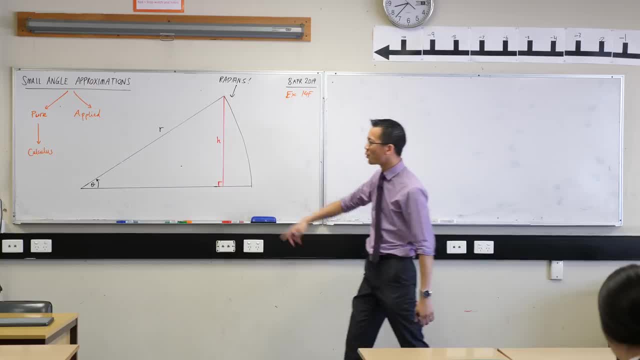 And you'll think: why are we doing this? It's some arbitrary thing. Well, all the results on which calculus of trig functions are penned, we're about to do this morning, And because they're based on radians, everything following this is also going to be in radians. 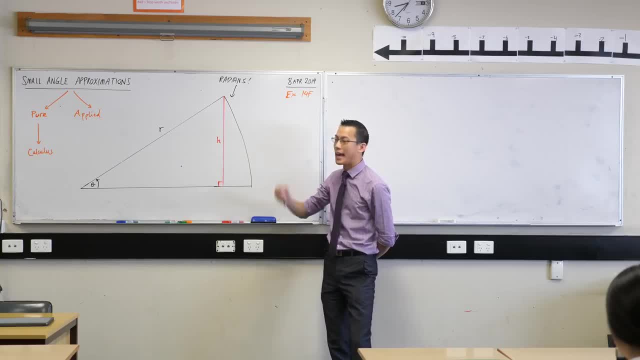 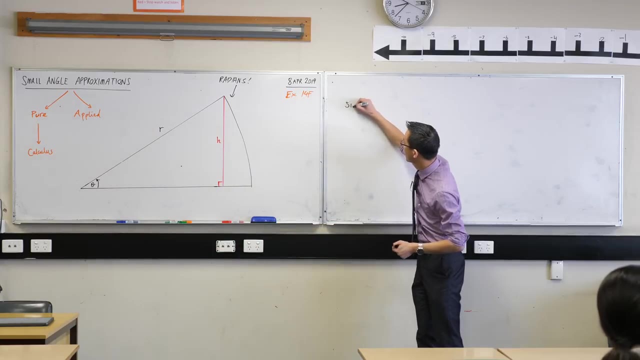 Now you guys know, in maths frequently we gain knowledge from looking at a single object from more than one perspective. Think back to auxiliary angle. You guys have already covered auxiliary angle, right? So the whole idea is: if I give you a function, 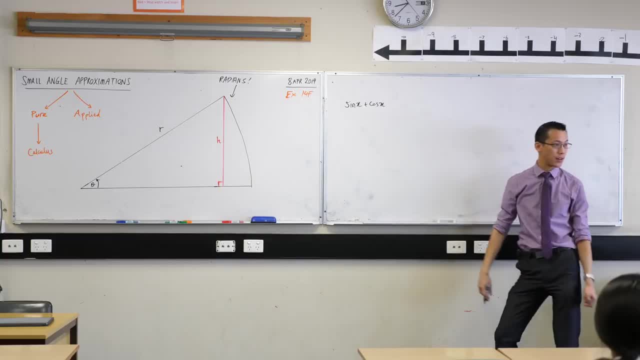 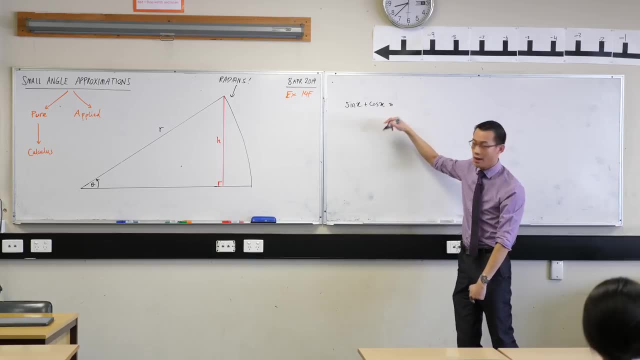 that is the sum of two other trigonometric functions. you can write it in a new form. You can say: okay, I'm going to have a new wave function out of these two. It's going to have a different amplitude And it's also going to have a different. 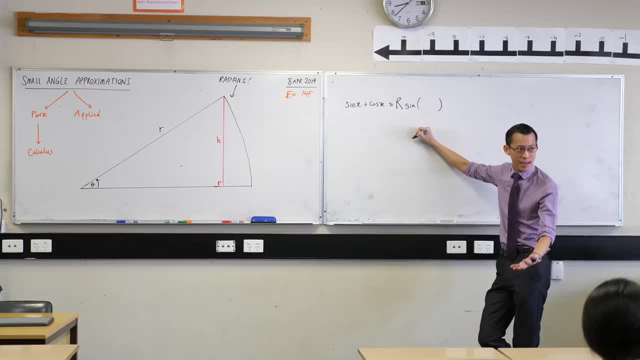 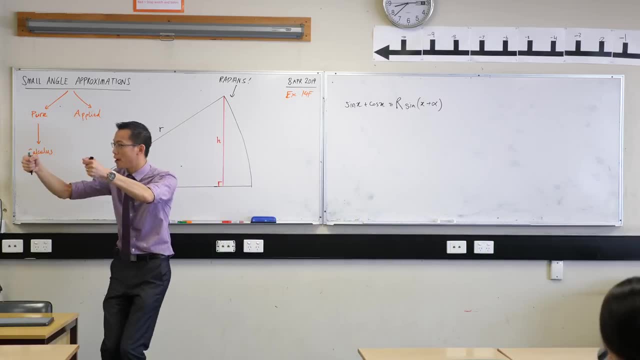 what's the other thing that's going to change? It starts with a P. Have you guys learned this word yet? It's going to have a different phase. Thank you very much. So when you take your wave function, it's the same wave function, same amplitude. 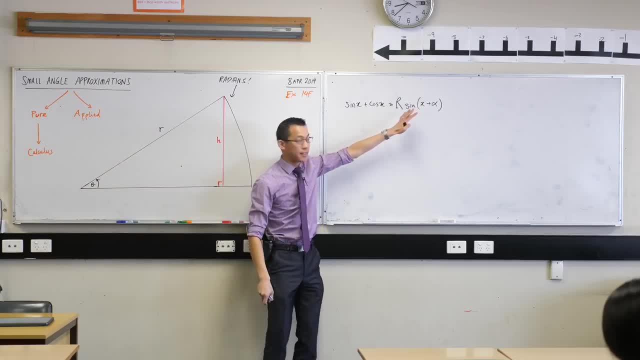 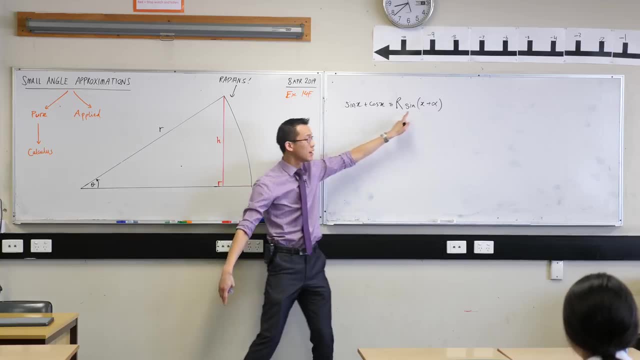 but if you shift it along horizontally, we call that the phase. Now, these are the two same thing, They're the same object. Right, And I like this because you're like, oh, single trig function, I can deal with this much easier. 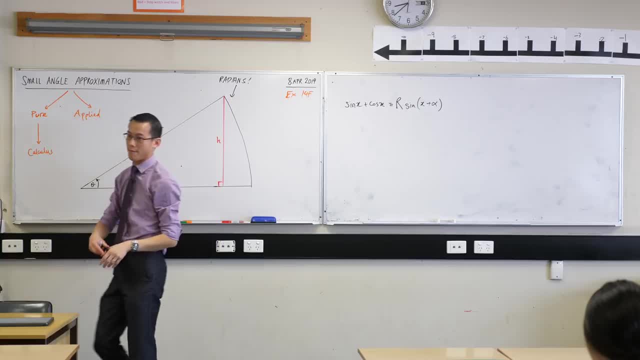 So you've got the same object looked at from two different angles and you gain insight, Right, And we're going to do exactly the same thing within this diagram And you can see the object I'm interested in, because I've highlighted it with color. 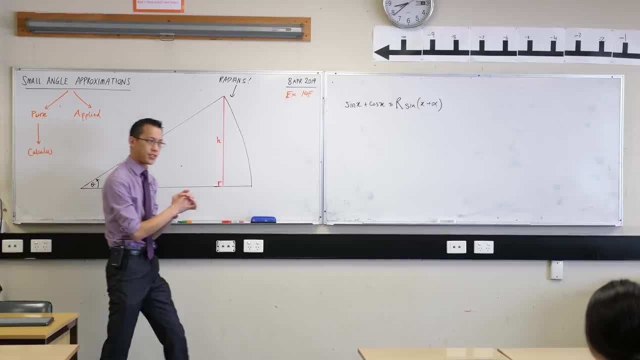 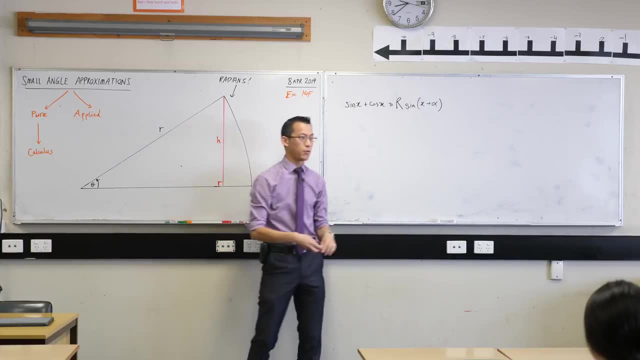 Right, This H here is what we're interested in, and we're going to look at it from two very simple perspectives and therefore gain some information out of this. Now, I've deliberately left some stuff off here which I want you to add along with me. 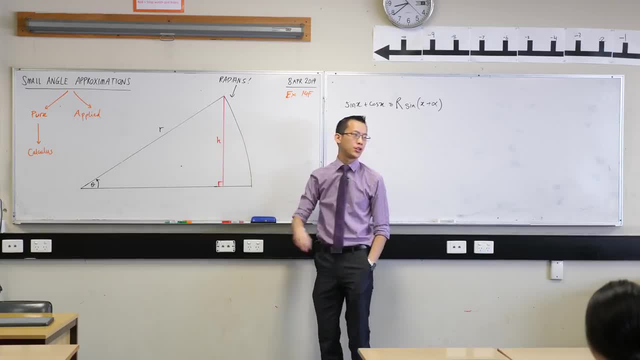 Okay, To get at this H over here, to look at it from two different perspectives. I want to focus on this guy down here. See this little length between our vertical length and our arc over here. This guy's going to be important. 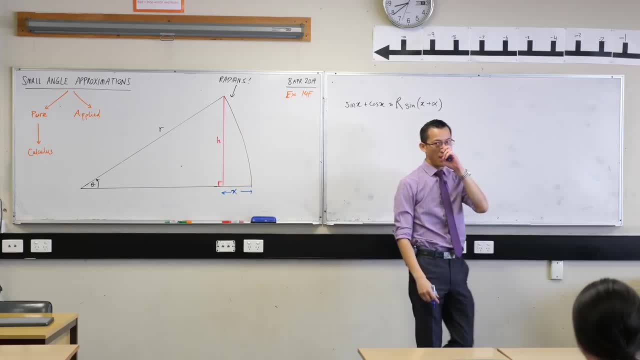 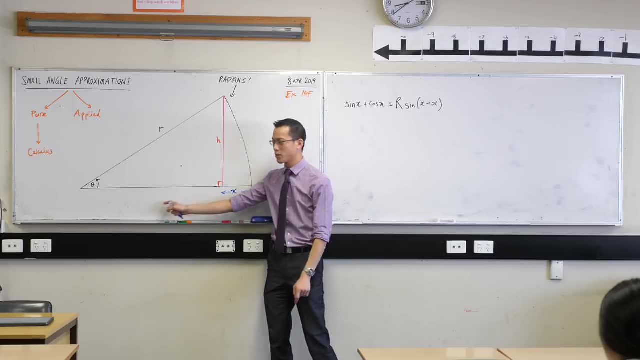 so we're going to call him X. Right, That little length is X. Now, because along the bottom here this is the edge of a sector. if this is X, what does this remaining length end up being R minus X. 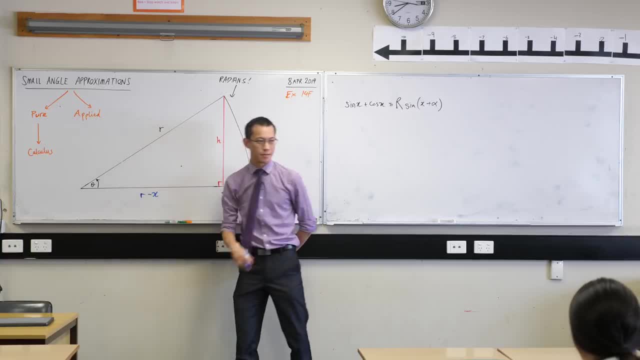 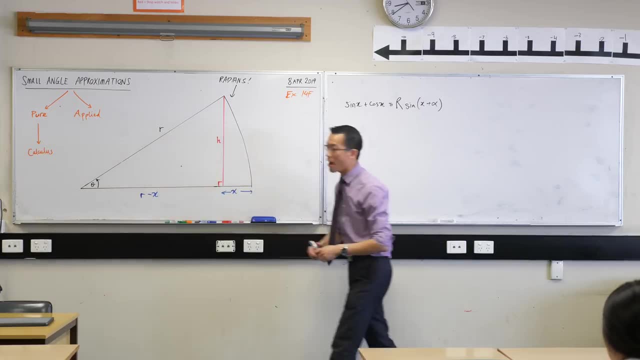 Right, It's just that difference there. Okay, So far, so good. I've done all my setup. Now I'm ready to actually understand this thing. That red object there, that's the H. It exists in a right-angled triangle. 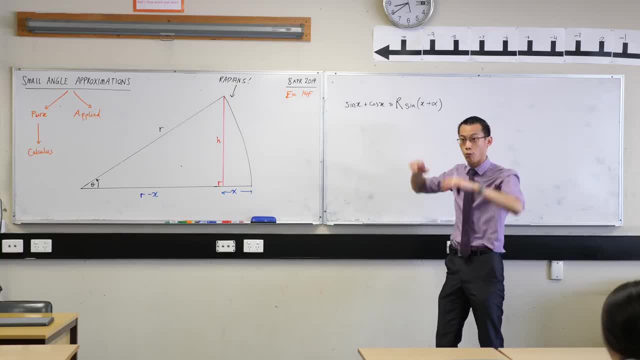 and I know that angle that's subtended at the center of this big circle of which I haven't drawn the whole thing. So therefore, I can state H in terms of, well, in terms of a variety of trig functions- I've got three to choose from. 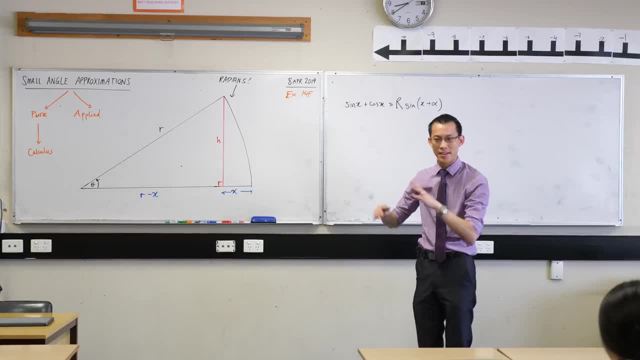 but I'm actually going to be, for reasons clear. in about 10 minutes I'm only going to focus on sine and tan. Can someone tell me what statement can I make with H that has sine in it? I'll give you a clue. 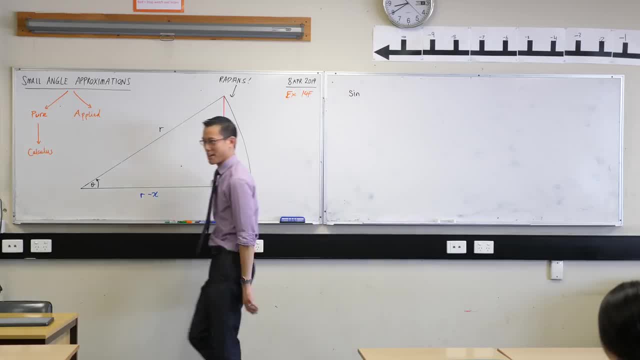 It starts with sine. Tell me what I can write next. You've only got one angle in this triangle, right, So maybe I should take sine of Theta. Wow, It's almost as if I've given you information that leans you in this particular direction. 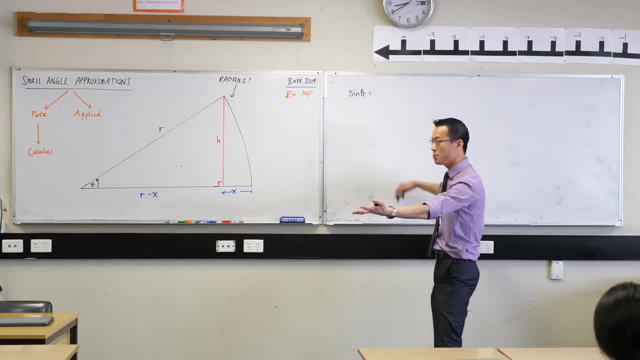 In this right-angled triangle, sine theta, of course, is equal to Opposite. on hypotenuse, Okay, Now this is true, but remember I told you, the object I'm really focusing on is actually that H right. 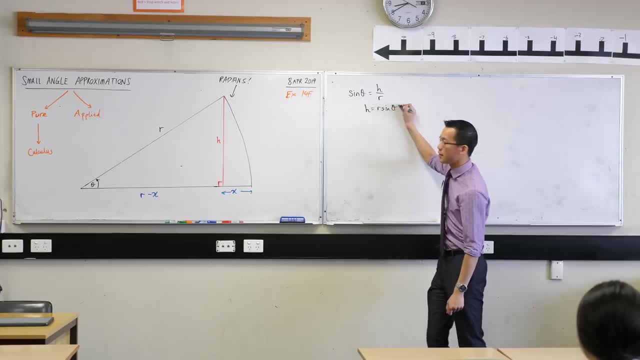 So I'm going to change the subject here and I get H equals R sine theta out of that. Are you so far, so good? Okay, So I have a statement for the length of H, but that's not the only perspective from which I can look. 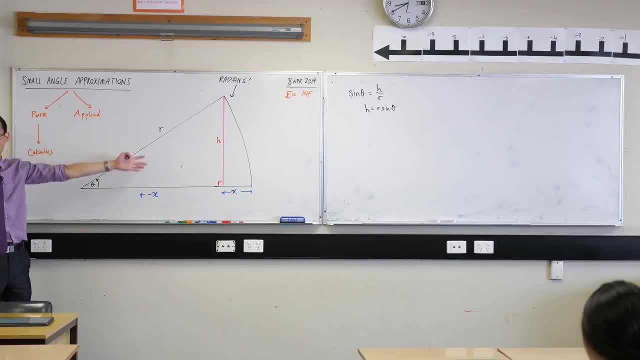 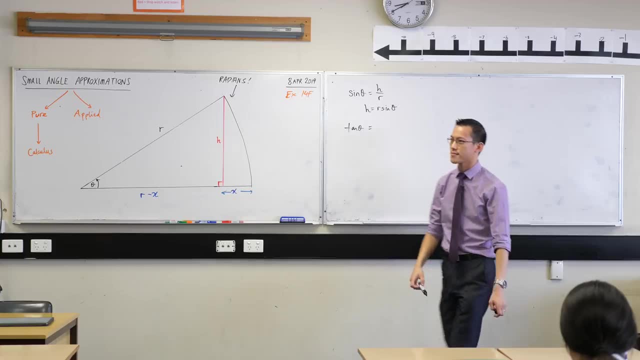 I'm going to write a statement with tan in it. I'm going to give you a second. You go ahead, You write it down. I'm not going to do it together. You guys can work this part out. Okay, Chester, what have we got? 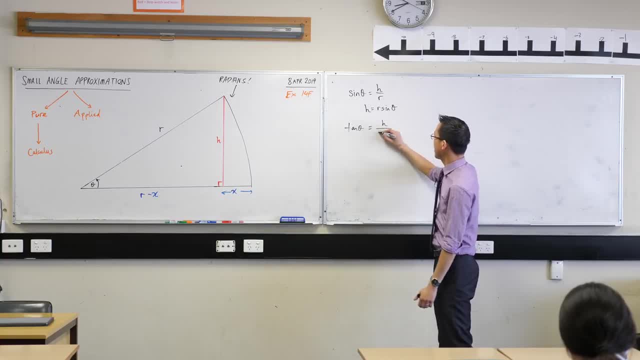 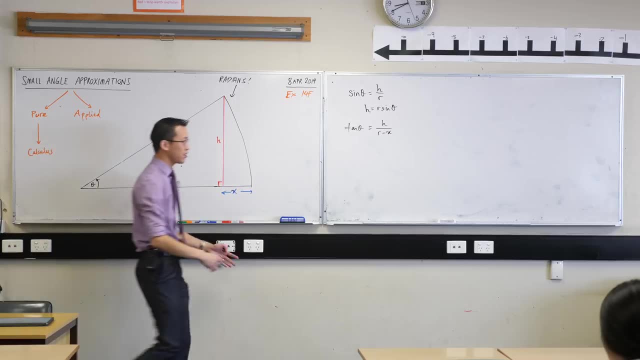 Equals to H over R minus X. Okay, So this is H on R minus X, opposite on adjacent. All fine, But again, remember, the thing I'm really interested in is H, so I'm going to change that to be the subject. 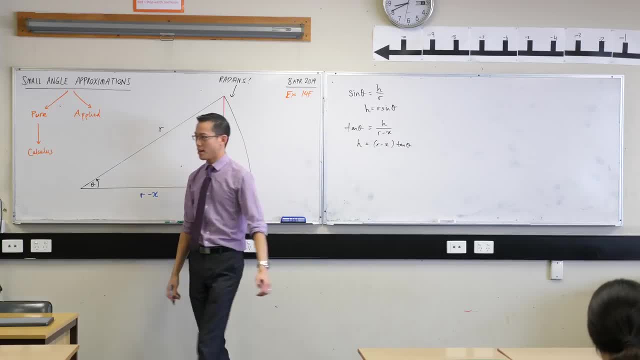 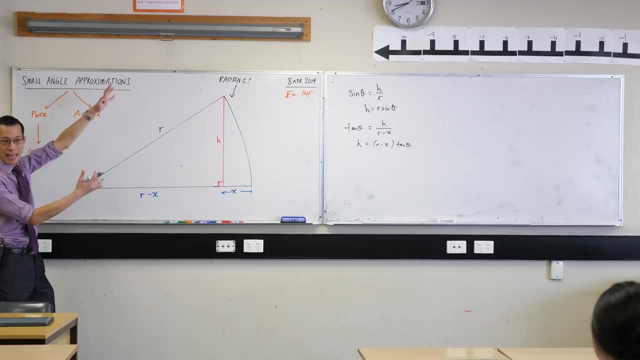 and this is what I get. Okay Now, nothing particularly groundbreaking so far. but you notice that I have the same length H and set it in two different ways, so I can actually equate those right. I can say therefore: 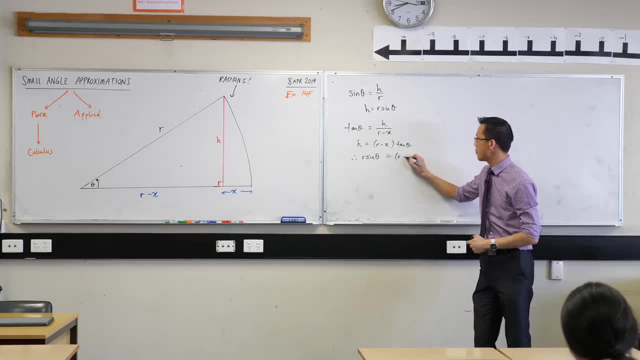 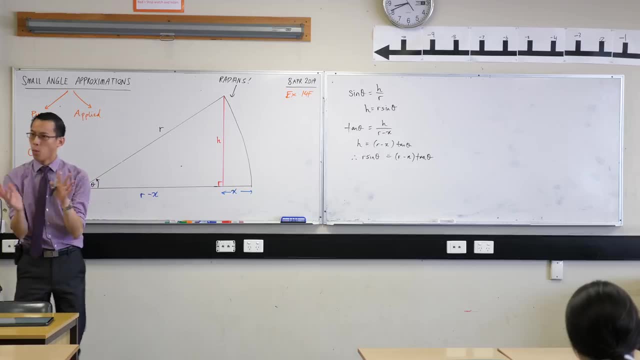 R sine theta and R minus X tan theta. these are the same thing, just looked at in two different ways. Okay, Now why would I bother doing this? Well, see my diagram. See how it's so comically large, right. 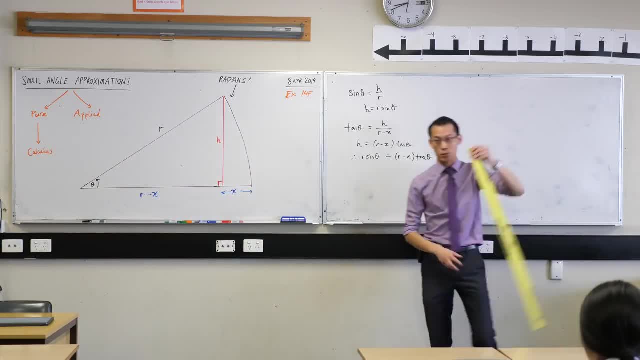 The reason it's comically large is because I use this meter rule for this very specific reason, okay, And if you've got your ruler there also, I'm going to pop it down here. I'm going to pop it down the end here. 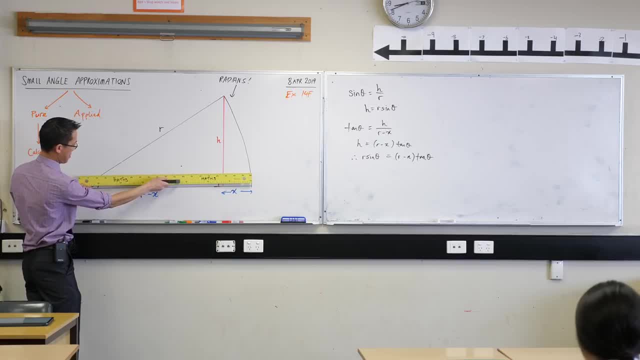 just so you can see all my. Actually- no, I'll put it on the top. You can still see my X and my R minus X. there, There we go. There's one. There's my radius in yellow, and then here's my other radius. 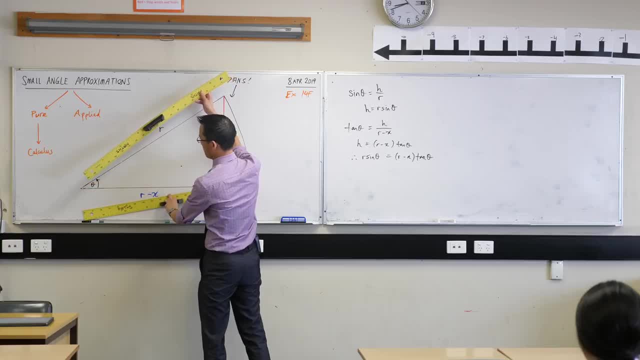 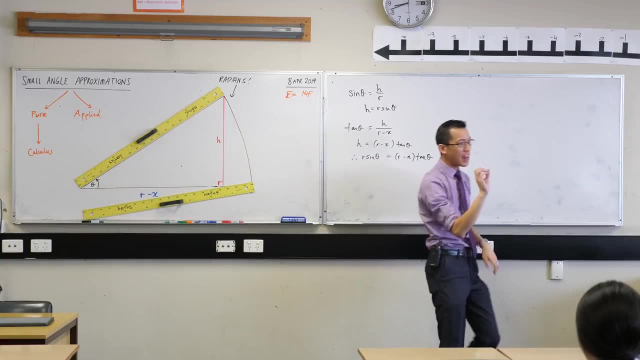 Now what I've got here- No, I am going to have to put it lower. What I've got here, That's better- Are these two radii, and I'm interested in what happens when the angle gets smaller, hence the heading. 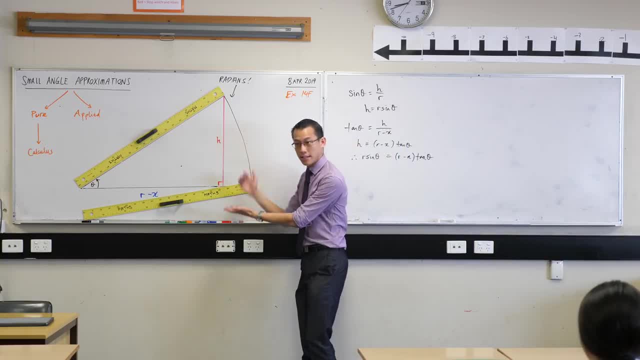 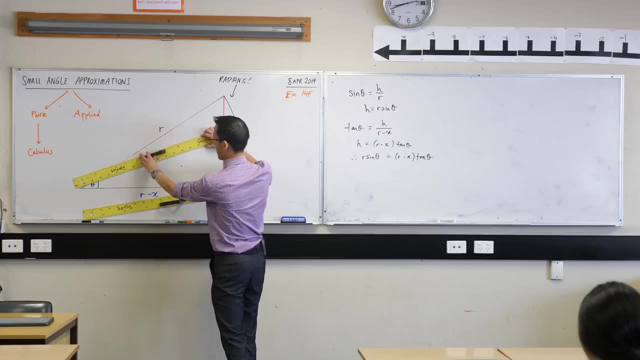 small angle approximations: okay. So as theta gets smaller, as it shrinks down, okay, this radius is not going to be up here anymore. It's going to be at spots like say that, There we go, That'll do me. 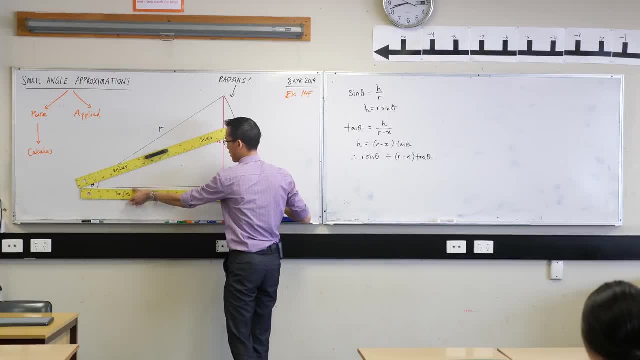 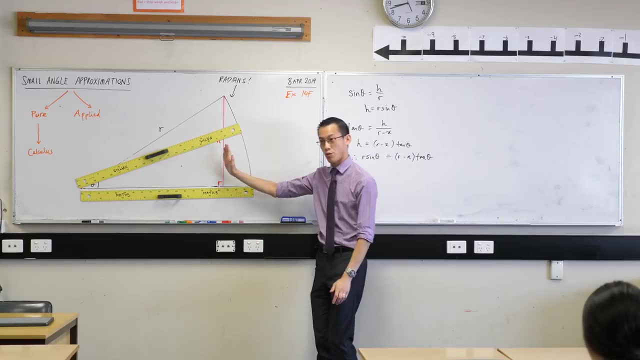 Okay, Now can you see as theta gets smaller, this is like theta. okay. What's going to happen is this? H is going to change, isn't it? Its position has changed entirely. It's going to be moved over here to the right. 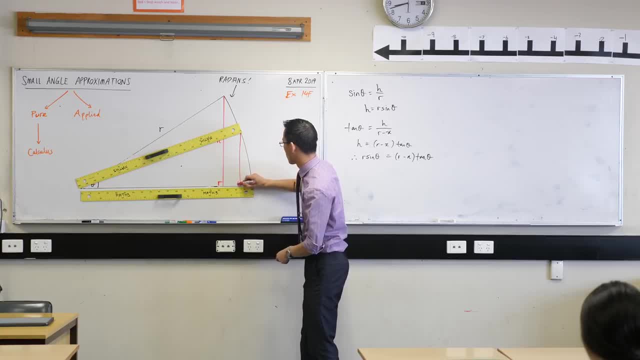 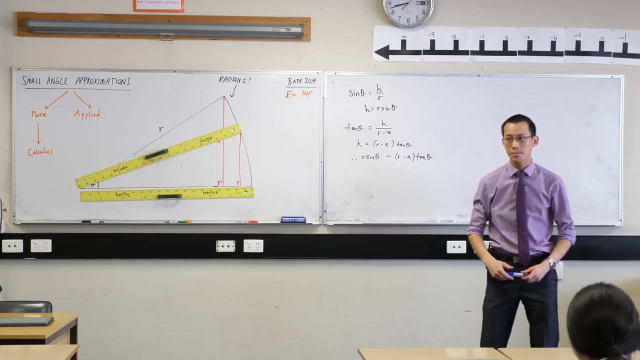 so it's going to be like. so You might like to put this in as well. Okay, I've got a new H, but along with that new H, I also have a new X. Where is X in this diagram? Have a look. 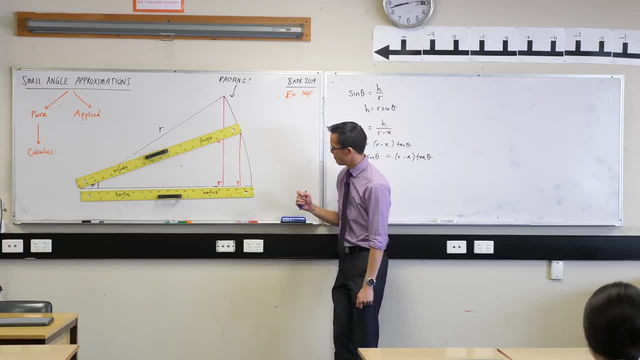 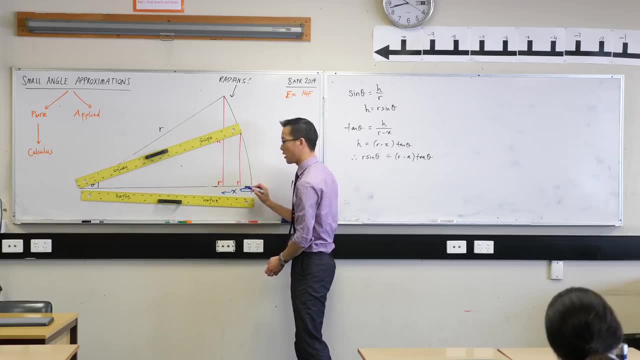 Where would you place it? It's just like teeny tiny little length over here, right, And that's actually very important that it's getting teeny tiny, this new X over here. You can see as theta gets smaller as I move this radius down even further. 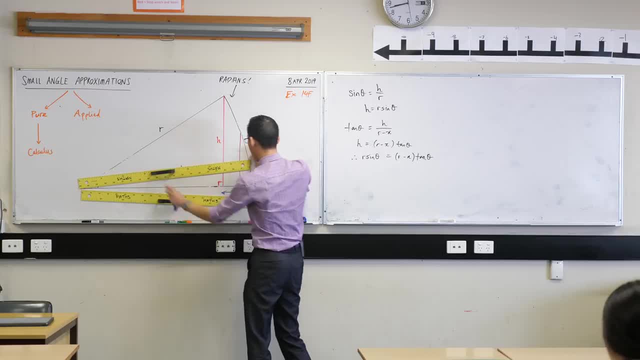 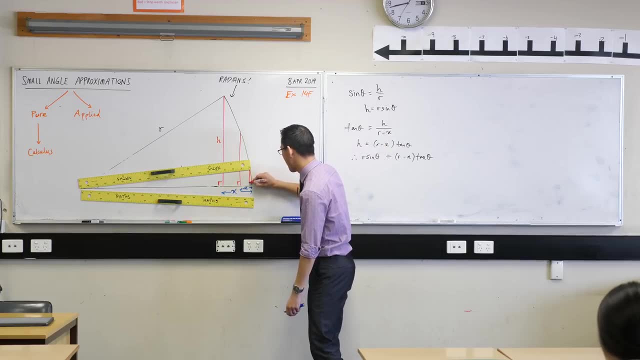 let's go down like this. In fact, at this point here I'm going to draw one more, and probably on your diagram you'll not have much space to do any further than that. Like that, As theta gets smaller, what's happening to X? 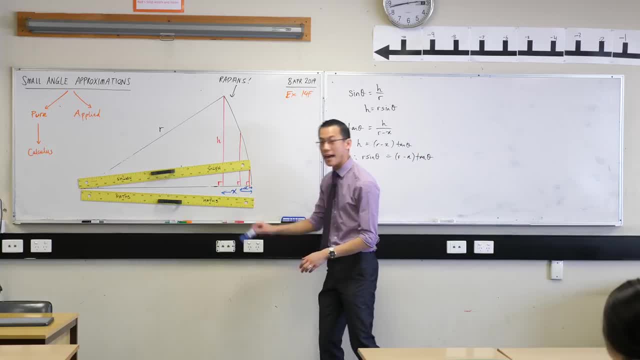 It's just vanishing away, right, As theta disappears. as theta approaches zero, so does X. So I have a way of stating this: right, Wrong colour, I can say, using my language of limits: right, I can say: 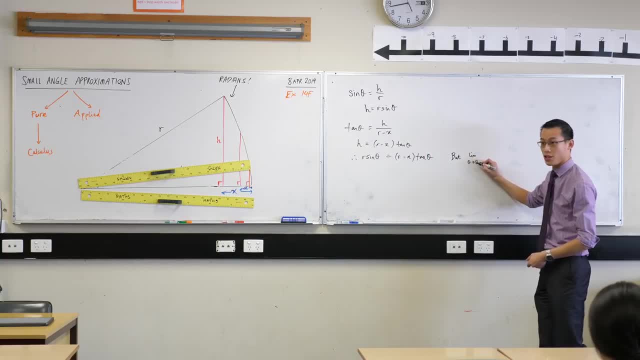 but the limit as theta approaches zero of that length X. what is that limit? What's it approaching? What did we just establish? Also approaching zero, right? So, therefore, if I think about this in the context of this statement, 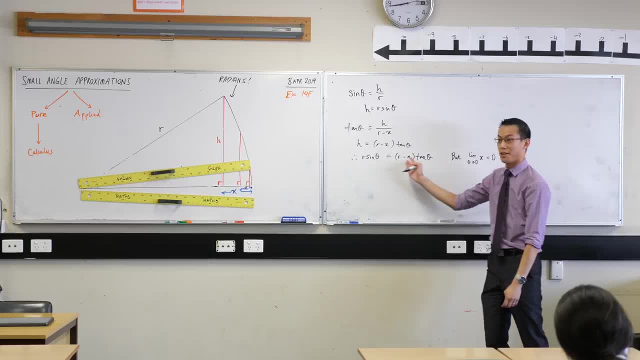 that we just made over here about H. right, We've forgotten that it was about H. we don't need to know that. that's where it came from, but that's where we learned this right, Just simple. right, angle, triangle, triangle. 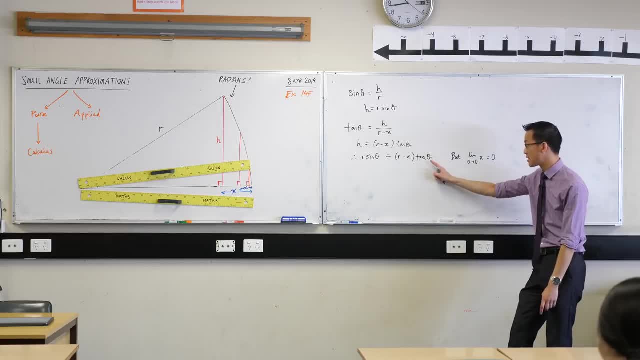 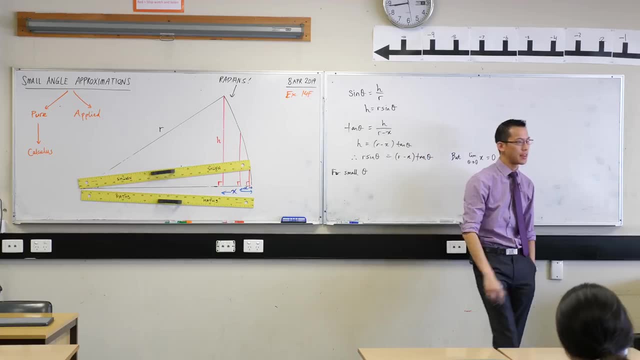 I can take the limit of both sides here. as theta approaches zero, right, In other words for small values of theta. this is what happens. when theta is approaching zero, We say: they're getting little right. I'm going to have R sine theta. 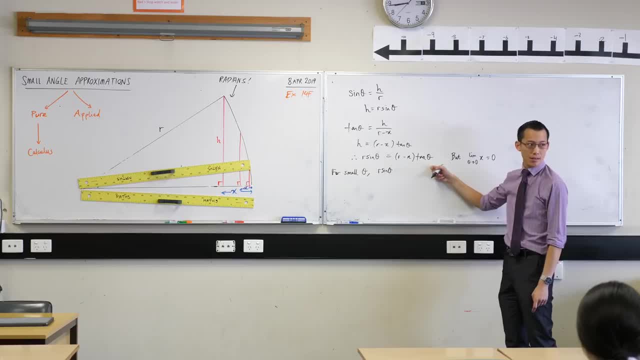 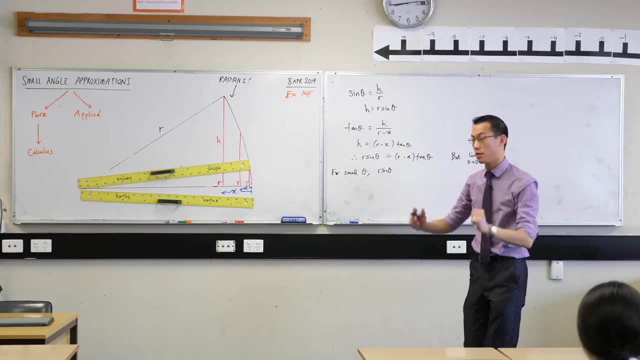 on the left hand side. What's going to happen over here? What's happening to that X? We just established this, right: That X is just vanishing away. It's just disappearing, right. So these things are going to become. 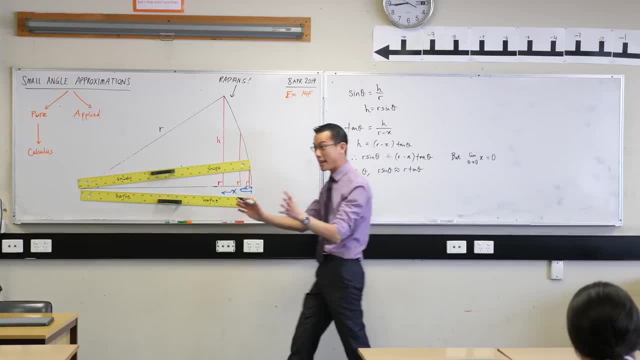 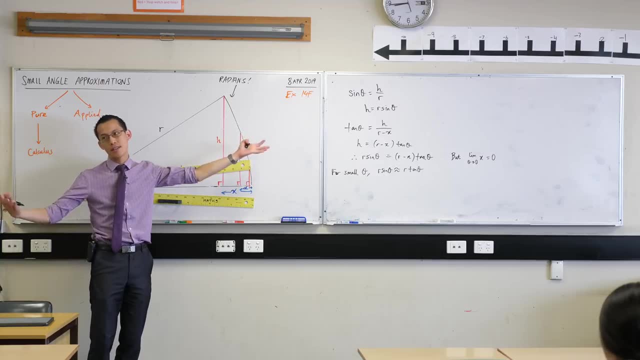 equal to each other. Without that X, you see what happened. That was like R minus zero and it's just vanishing away. okay, Now you can see here. R is just a length of any description, so I can divide both sides through by R. 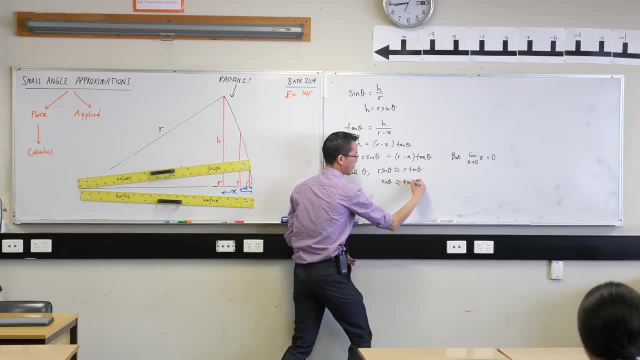 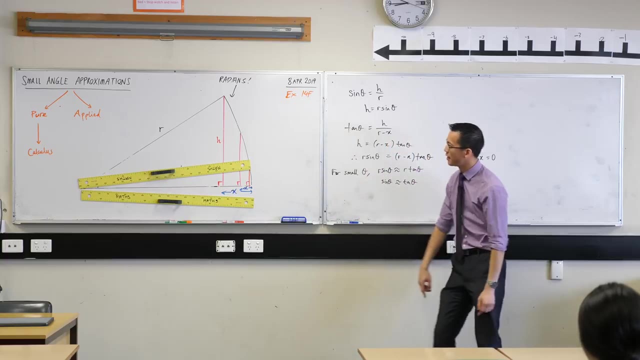 so I'm getting this Like: so okay, Now, sine theta and tan theta. what are we saying? As theta gets smaller and smaller and smaller, the difference between them is really this: X and that's getting smaller and smaller and smaller and smaller. 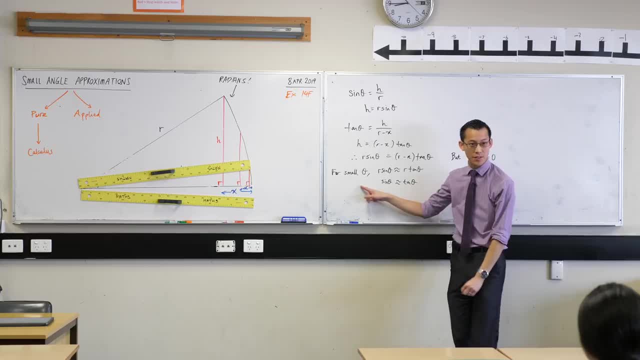 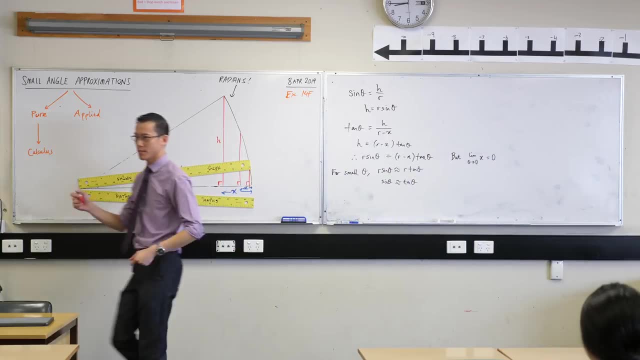 You can see that these things are approaching each other for small values of theta. What does sine theta actually approach when theta gets small? Think about the graph. What does theta- sorry, what does sine theta approach when theta itself gets small? It also approaches zero. 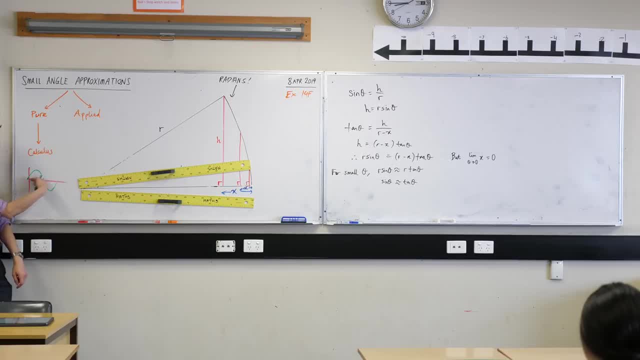 If you have a look at the graph there, right, As theta approaches zero, as it gets closer and closer into the origin, right? Do you see that theta is getting to zero? So is sine theta, right? What about tan? What does tan approach? 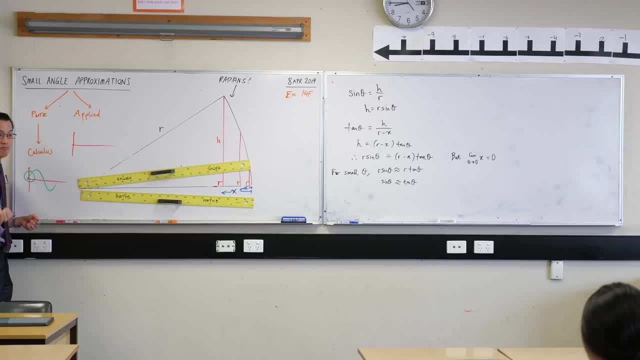 when you are getting closer to zero. Same thing right. Here's the graph. Actually not interested in this part over here, but this is so. you recognize it as tan And, as you can see, as theta gets closer and closer to zero.